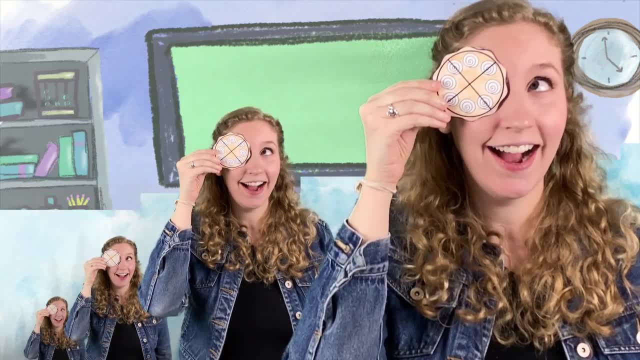 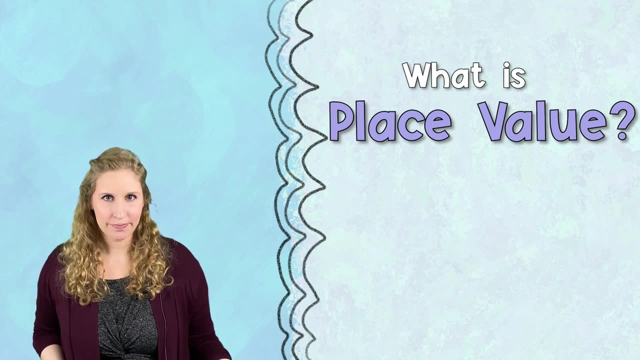 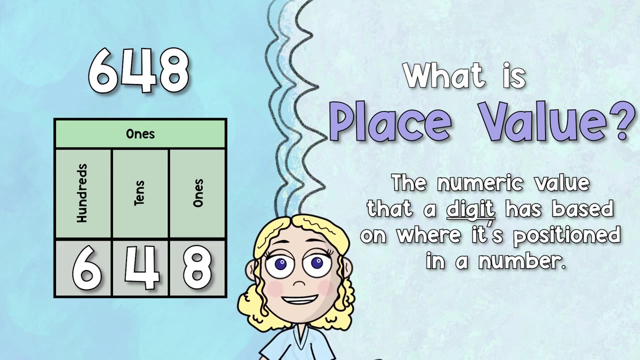 Area symmetry fractions too. It's all here for you, Alright. so what exactly is place value? Place value is the numeric value that a digit has based on where it is positioned in a number. Okay, so what exactly is a digit? 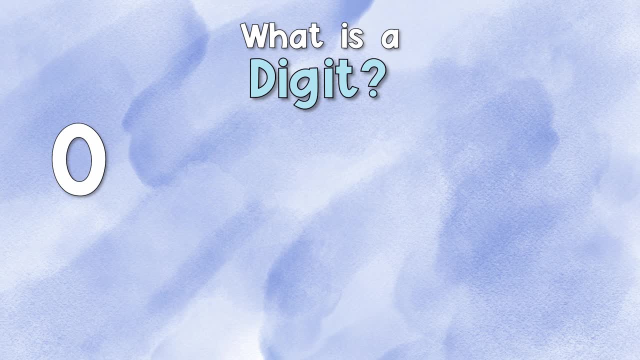 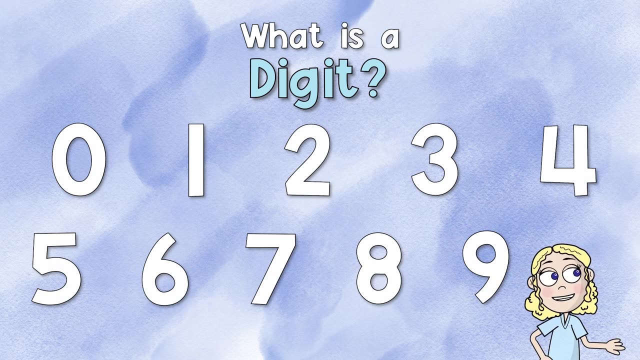 We have ten digits. Those digits are 0,, 1,, 2,, 3,, 4,, 5,, 6,, 7,, 8, and 9.. We use those digits in order to show what we have in each place value. 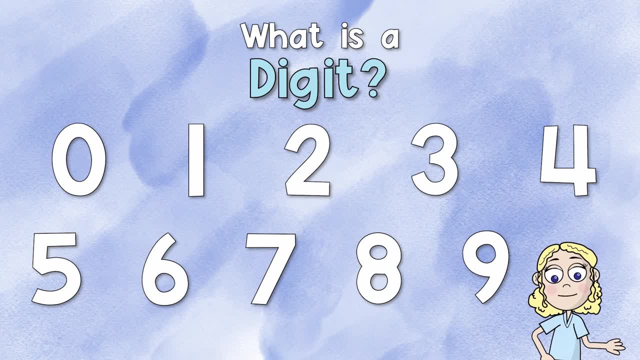 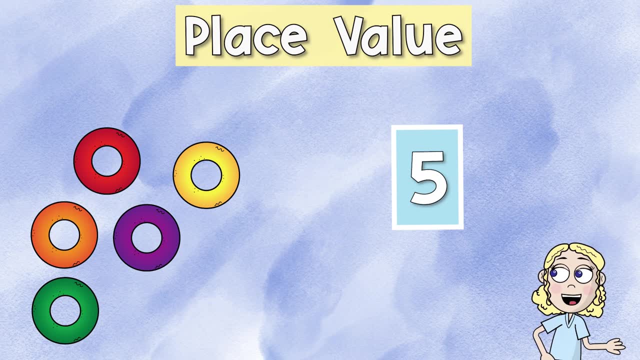 Let's look at this example right here. I'm going to have one cereal loop Alright when I get to ten: 1,, 2,, 3,, 4,, 5,, 6,, 7,, 8,, 9, and 10,. 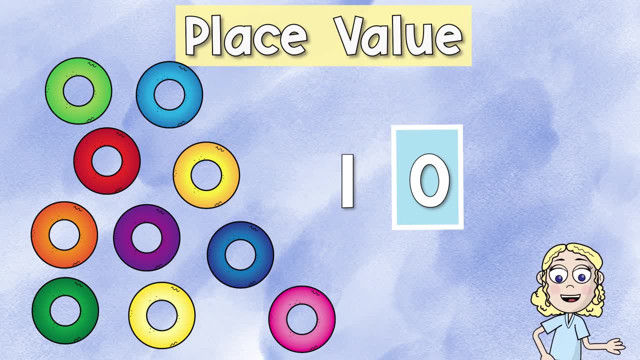 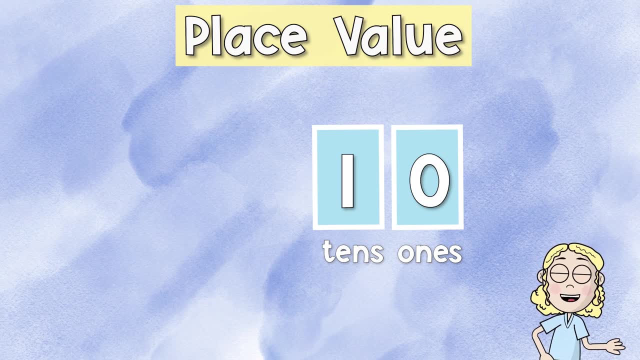 we actually run out of space in that place value and have to go to the next place value. This is the tens place. The tens place is going to show us how many groups of ten we have. So let's pretend this group of ten is right here. 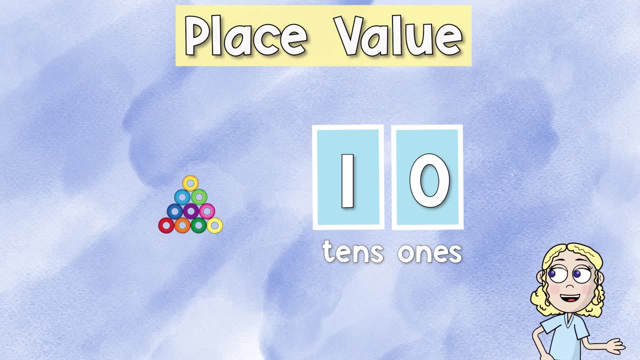 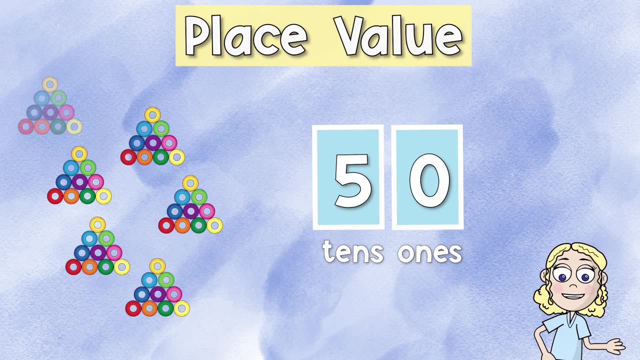 Alright, now let's count by tens. So in the tens place again we're going to go through each digit: 10, 20,, 30,, 40,, 50,, 60,, 70,, 80, 90.. 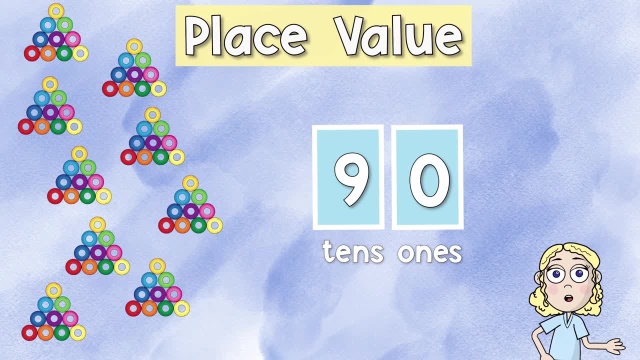 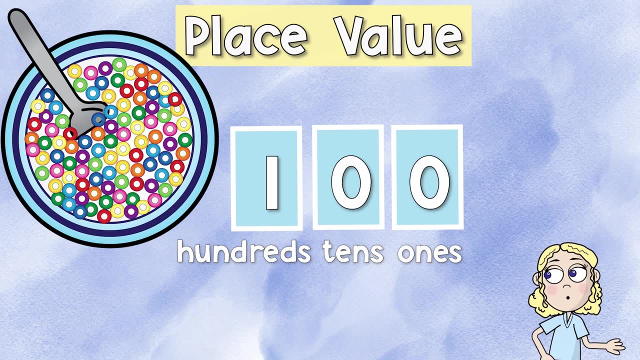 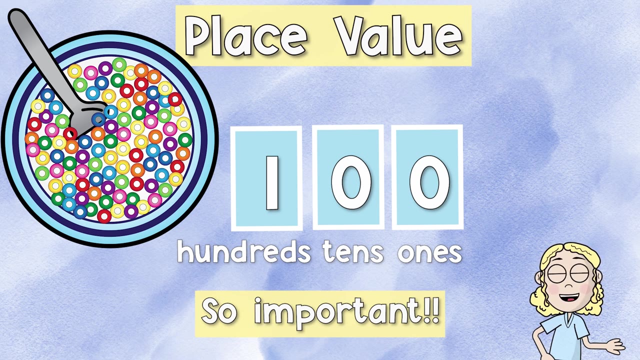 Okay, now what happens? There's no more room after 90.. We have to go to the hundredths place. So now we have one group of a hundred or one giant bowl of cereal. That's why place value is so important. It allows us to see how many groups of each place value. 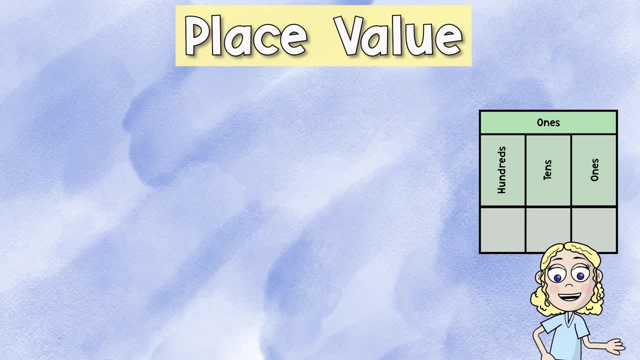 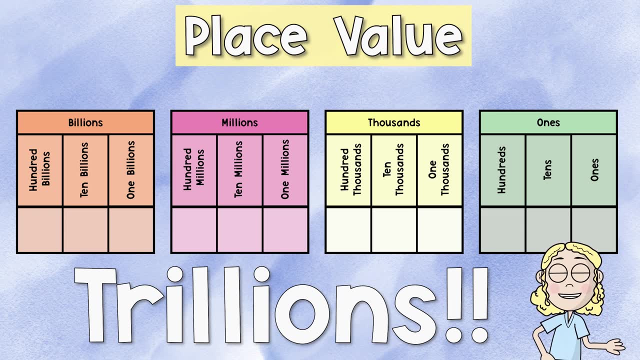 This also is the same thing That happens when you're talking about thousands, millions, billions and even trillions, Because you can get into super large numbers, And so when you look at something like this, you're thinking about how many groups of trillions you have. 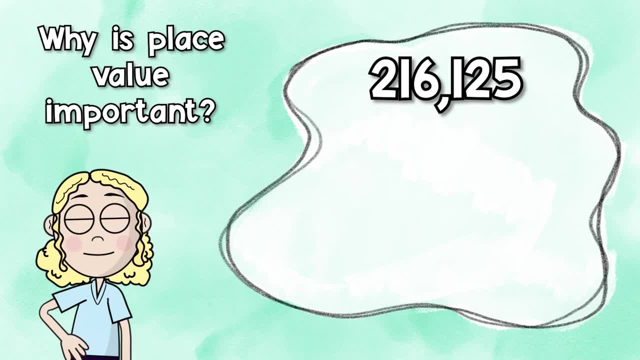 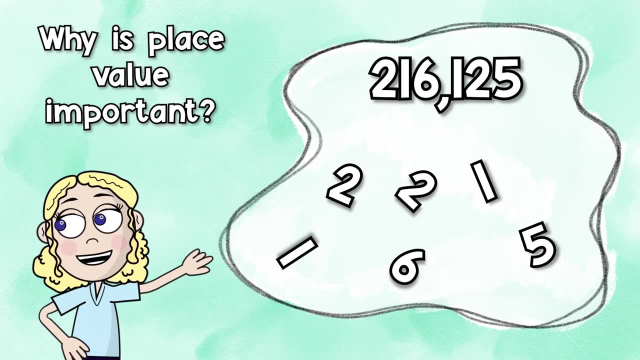 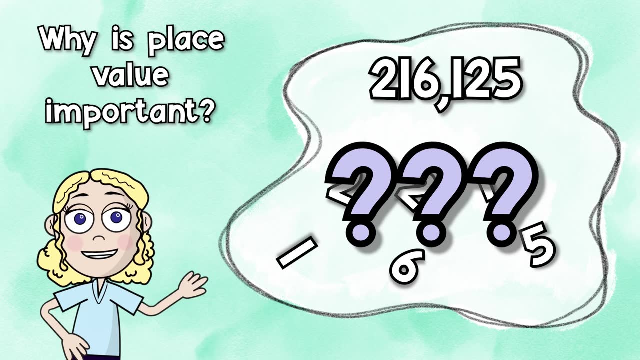 Why is place value important? Place value is important because when we look at a number, we'll know exactly what it represents. Imagine if we didn't have place value and we just put numbers all over the place silly willy. Then we wouldn't necessarily even know what represented what, and it'd be very confusing. 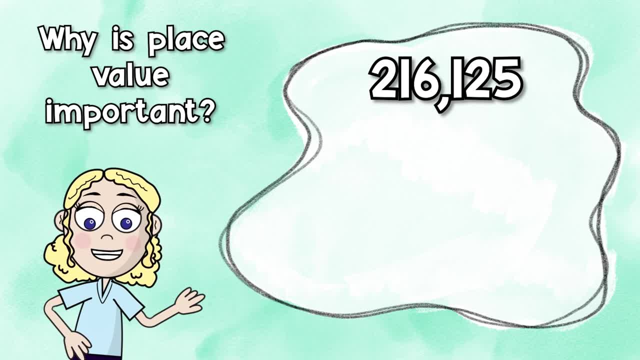 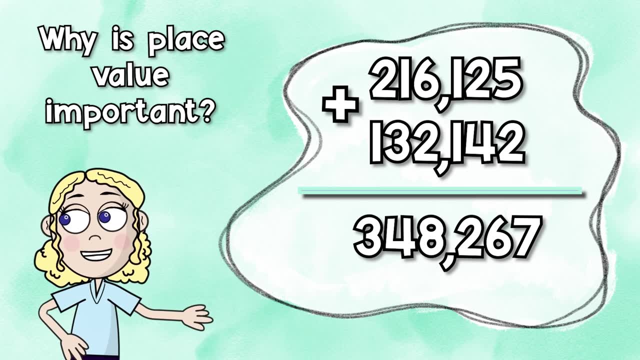 Another reason why it's so important is because when we do things like add, subtract, divide and multiply, we will know exactly what numbers and what value we are adding, subtracting, multiplying or dividing. It helps us compute those numbers, especially large numbers. 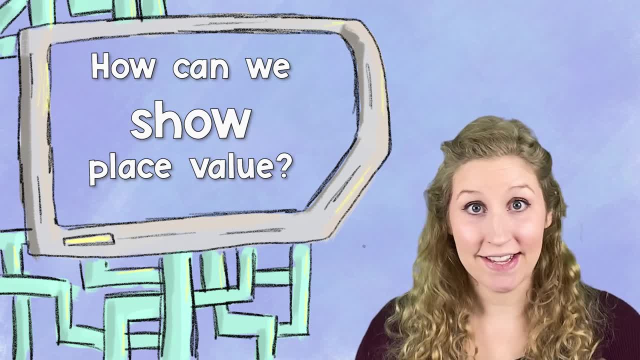 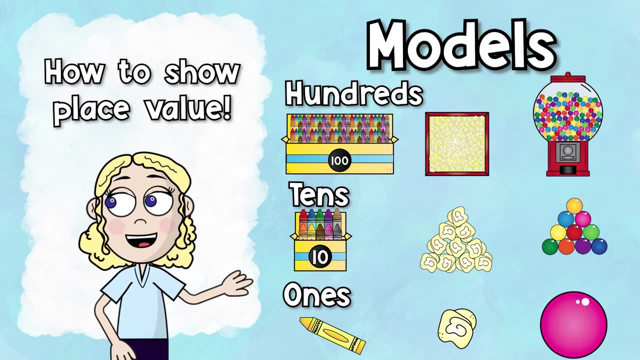 What are some different ways that we can show place value? You can show place value in a variety of different ways. You might have seen it look like this, where it's in model form, and there's a bunch of different types of models that you can show place value. 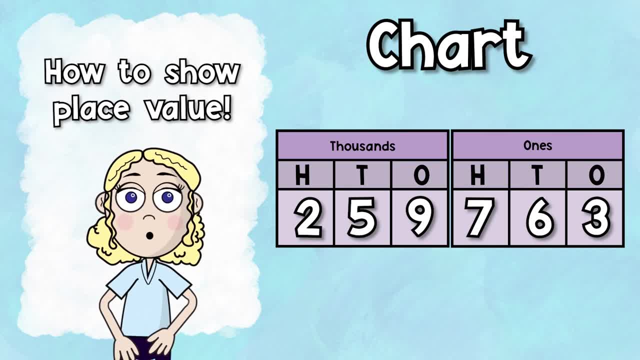 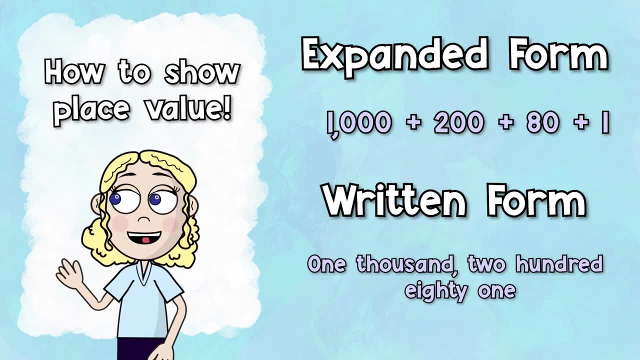 You might have also seen it in a place value chart, or even seen it in a couple different forms, like expanded form or written form. Let's take a look at a few of these bigger numbers and see if we can fill out a place value chart. 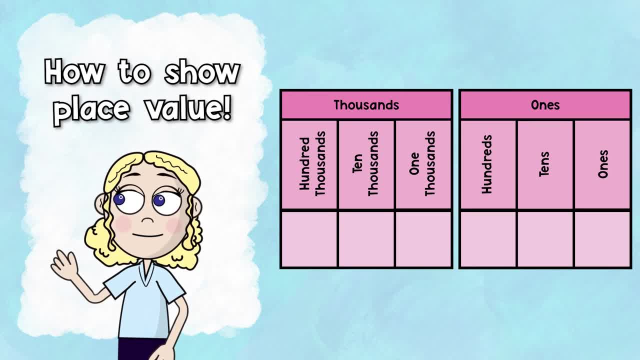 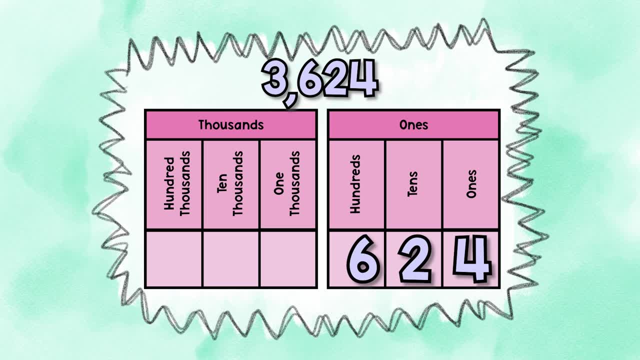 and see what the different place values represent: 3,600.. 224.. There's 4 in the ones place, 2 in the tens place, 6 in the hundreds place and 3 in the one thousands place. Let's try another one. 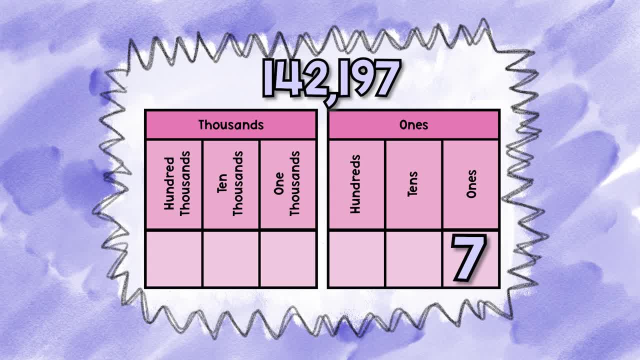 142,197.. There's 7 in the ones place, 9 in the tens place, 1 in the hundreds place, 2 in the one thousands place, 4 in the ten thousands place and 1 in the hundred thousands place. 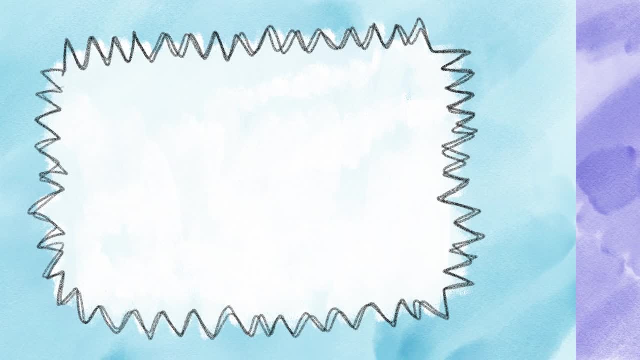 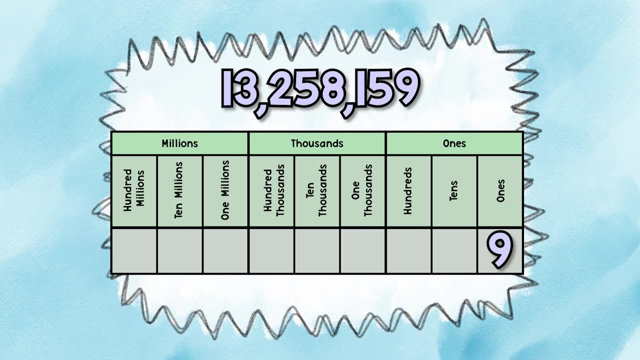 Alright, let's try a really large number: 13,258,159.. There's 9 in the ones, place 5 in the tens, place 1 in the hundreds, place 8 in the one thousands, place 5 in the ten thousands, place 2 in the hundred thousands, place 3 in the one millions place. 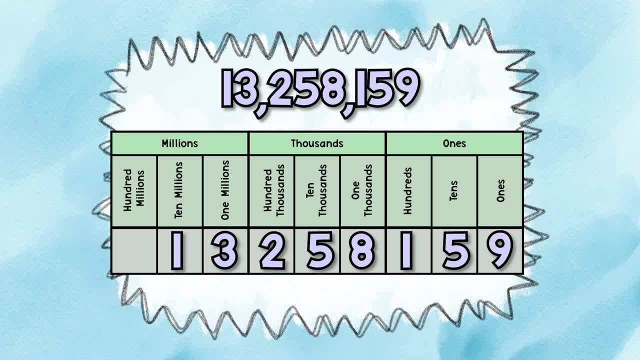 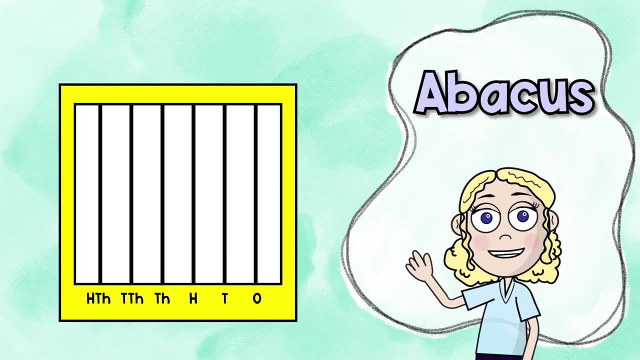 and 1 in the ten millions place. Did you get it correct? Alright, check this out. This is an abacus and this is actually an ancient way they used to not only show numbers but compute numbers. You can actually put place value on an abacus like this.